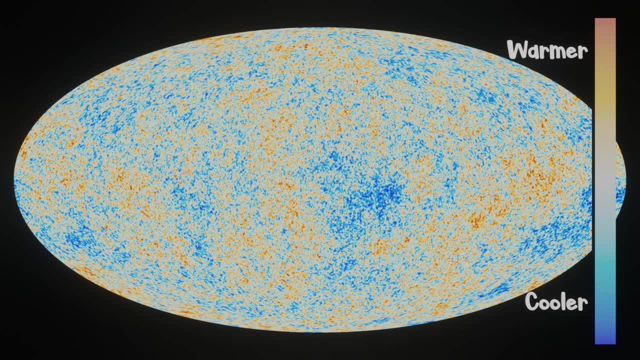 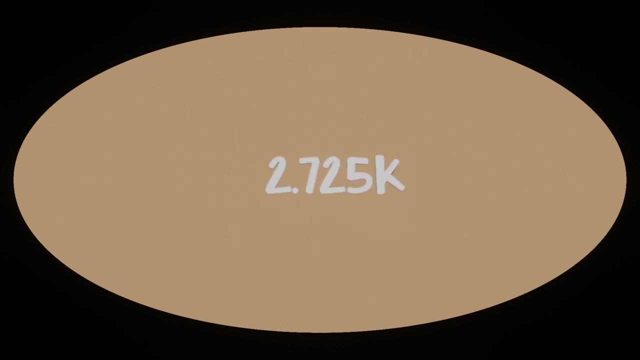 These colors represent temperature: red is warmer and blue is cooler, but we're talking on a scale of millidegrees. If you had an imprecise thermometer, it would all look 2.725 Kelvin. But this light tells us more than just the temperature of our universe or what was happening. 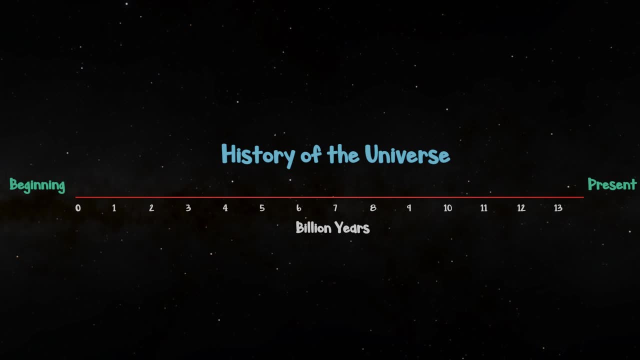 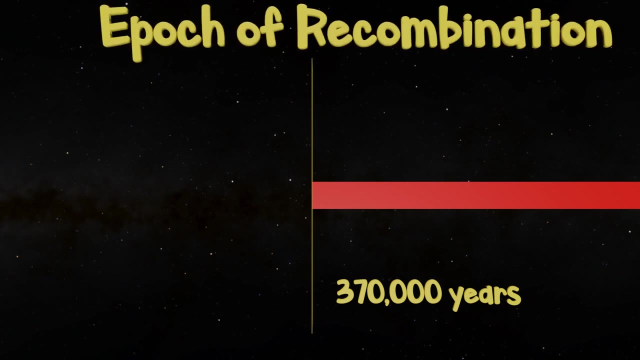 a long long time ago, Early in the life of the universe, a mere 370,000 years after its birth, a great event occurred in an epoch called Recombination. At this point, the universe had cooled down enough to allow electrons and protons to merge. 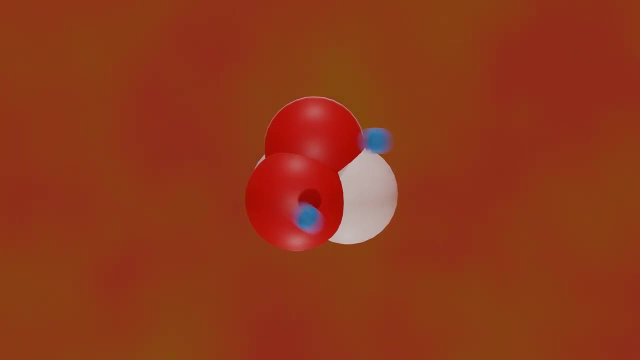 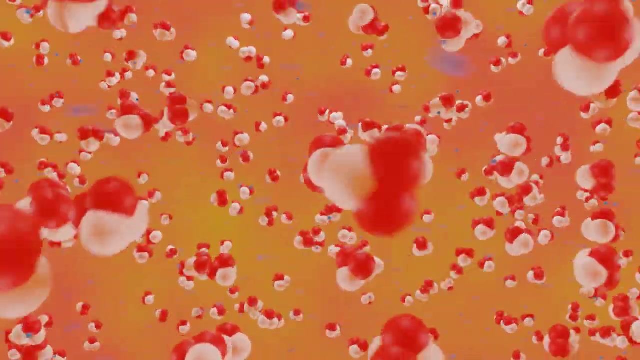 and form the very first atoms of helium. Prior to this, the heat of the universe was too intense. the energy held by individual electrons and protons was too great to allow them to remain bound to one another. This hot state, when electrons are not bound to protons, is called the heat of the universe. 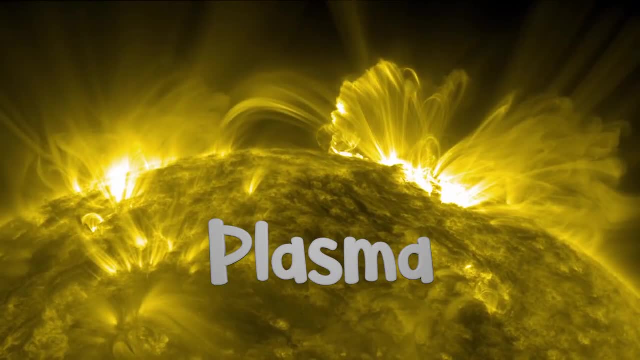 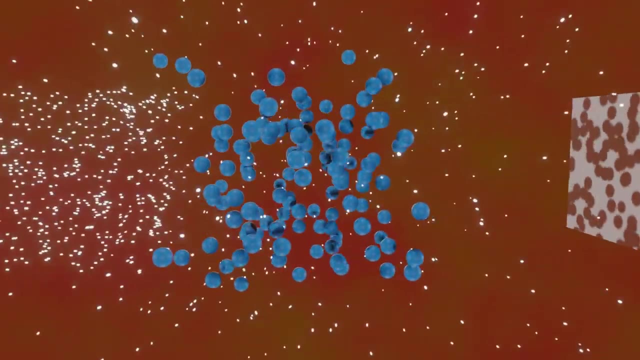 The heat of electrons is what we call a plasma like our sun. Because the electrons are not bound to an atom, they can freely scatter and interact with light. This means no light can travel in a straight line, thus no light could possibly pass through. 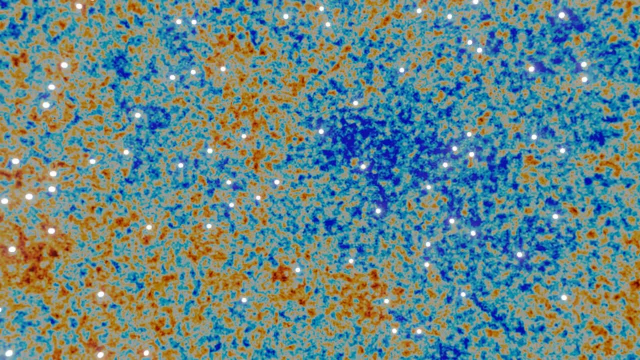 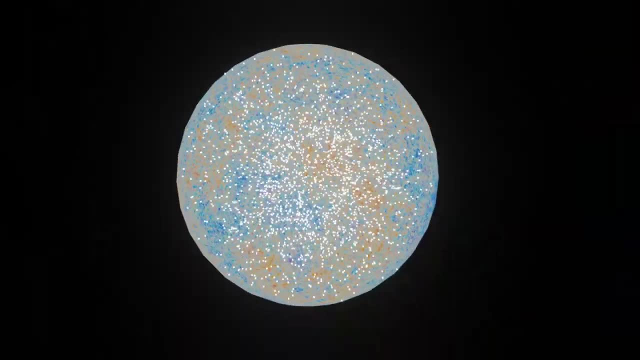 to form a meaningful image. What we do see, then, is the scattering and abundant release of light from this hot plasma, Kind of as if the wall was the surface of a star, And it's this ancient plasma that is creating what we call cosmic microwave background. 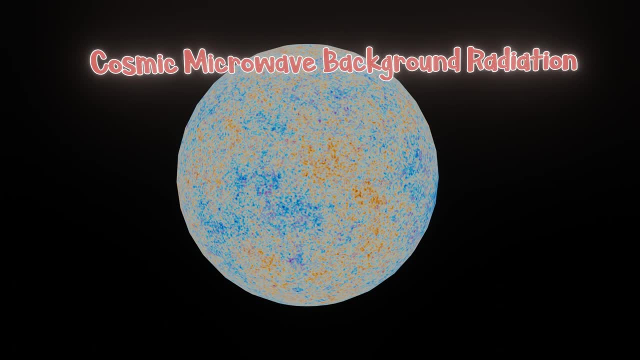 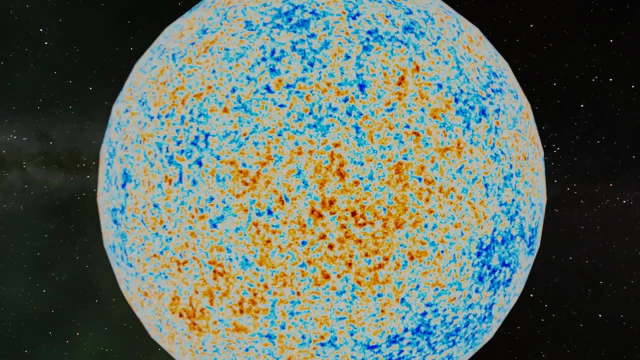 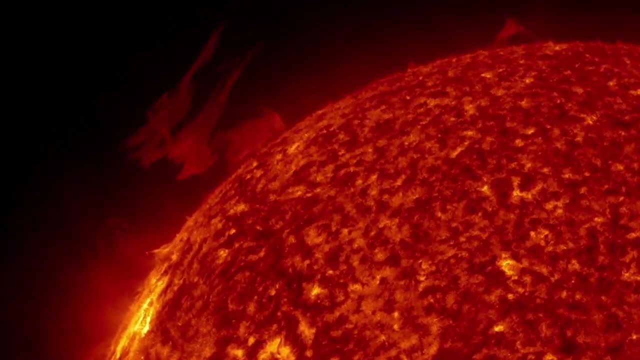 Now this may arise a few additional questions one may ask. So does this mean there is an edge to the universe, And are we in a sense inside a giant star? And if the light really does come from plasma, something we find in stars, why is it so weak? 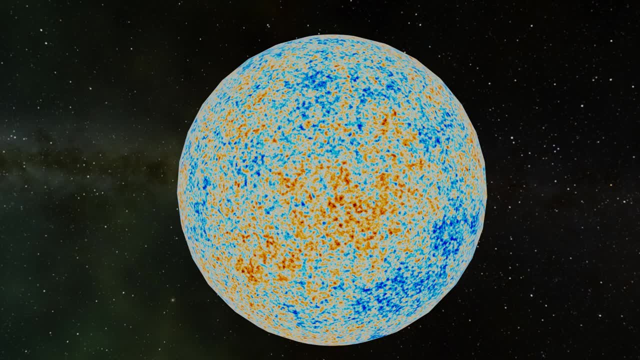 The first answer is that this is, of course, not the edge of the universe, And we can easily understand this visually. During the epoch of recombination, almost all matter was made of plasma. The first answer is that this is, of course, not the edge of the universe. 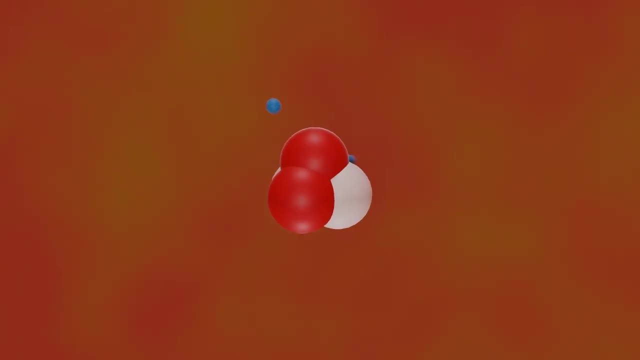 And we can easily understand this visually. During the epoch of recombination, almost all matter was made of plasma, And we can easily understand this visually. During the epoch of recombination, almost all matter in the entire universe condensed into helium at more or less the same time period. 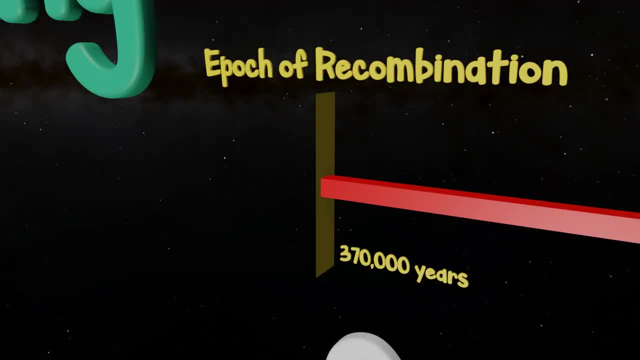 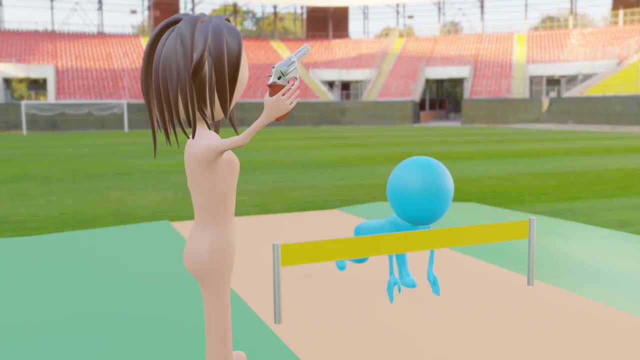 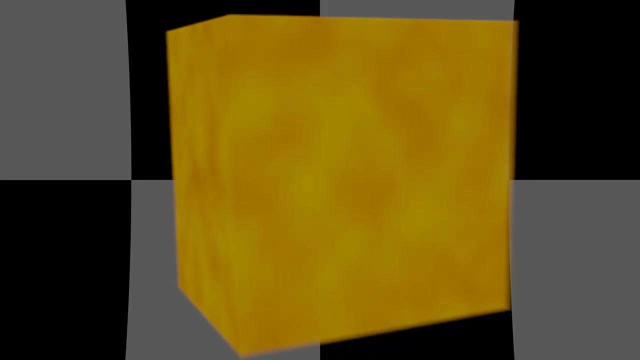 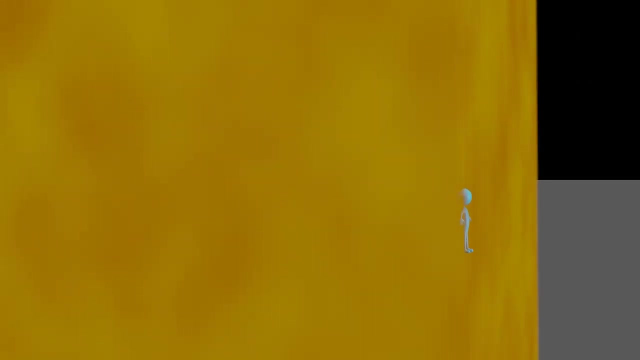 We the next transparent gas. However, for an observer within the universe, their observations are reliant on light, and light is very slow. So although the entire universe, at roughly the same time, became transparent, our observer would only receive this information as an expanding. 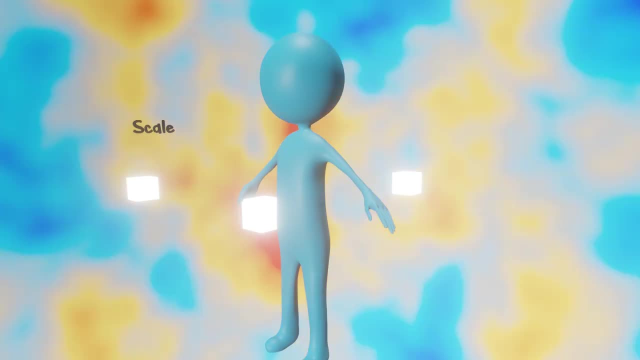 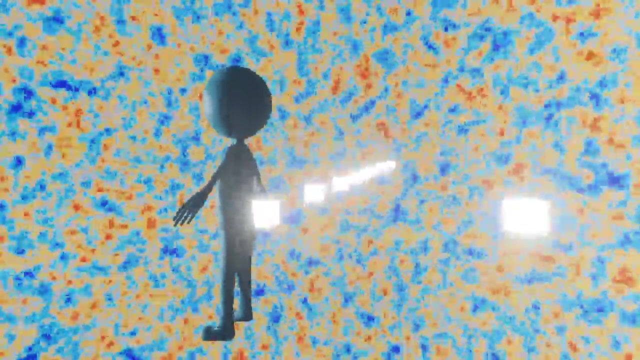 sphere that moved away from them at light speed. Wherever they looked, they would see ancient plasma that no longer existed, just like how we see ancient stars that also no longer exist. Now, here is where the truly bizarre implications begin. If we are seeing ancient plasma, 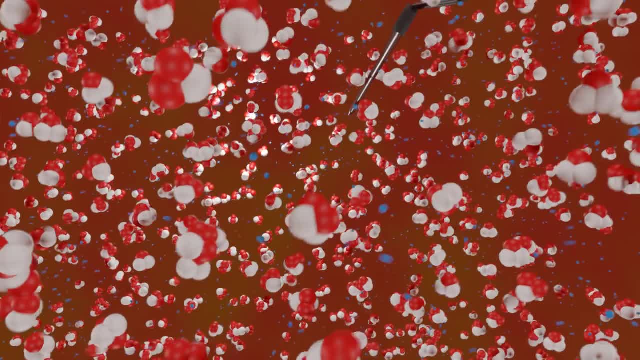 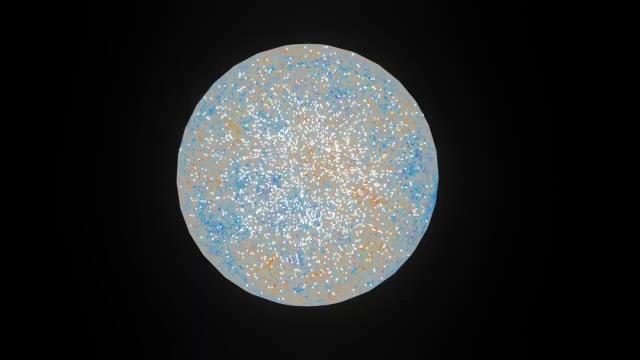 well, we know that plasma is really hot. In the conditions of the early universe, electrons and protons would not have condensed until around 3000 Kelvin, So the light emitted from this plasma should be in the visible spectrum. yet, as the name suggests, it's microwave light. 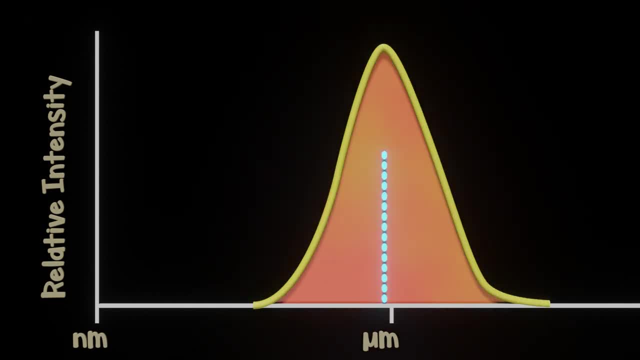 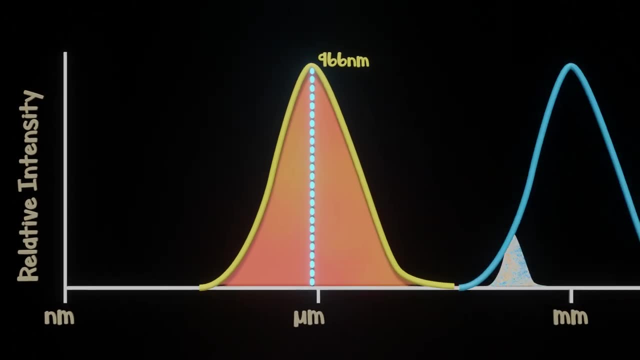 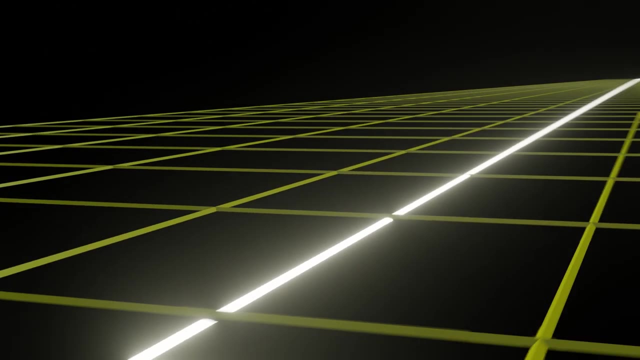 The peak wavelength from a 3000 Kelvin object should be 966 nanometers. We'll round it up to 1 micrometer, Yet the observed peak for cosmic background radiation is 1 millimeter. That means this light has been stretched out over a thousand times its length, And this is really strange. 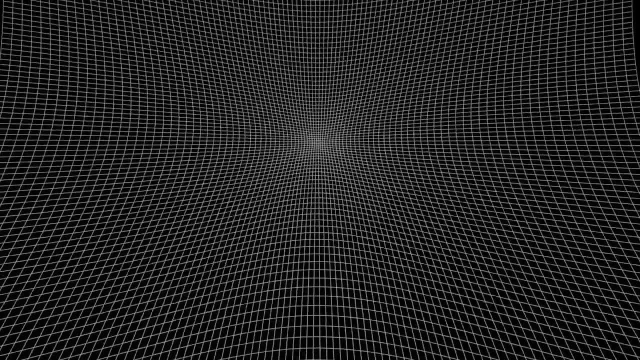 This stretching of our cosmic radiation is a result from spatial expansion. But this is a bit odd because, as far as we can tell, the solar system has always been a little bit more advanced. But this is a bit odd because, as far as we can tell, the solar system has always been a little bit. 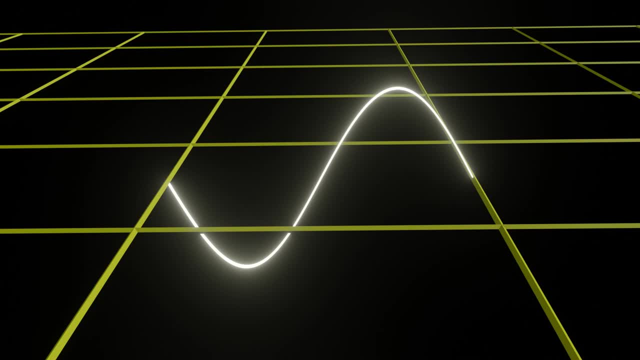 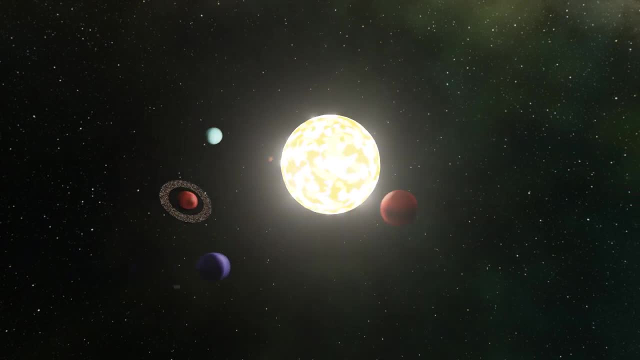 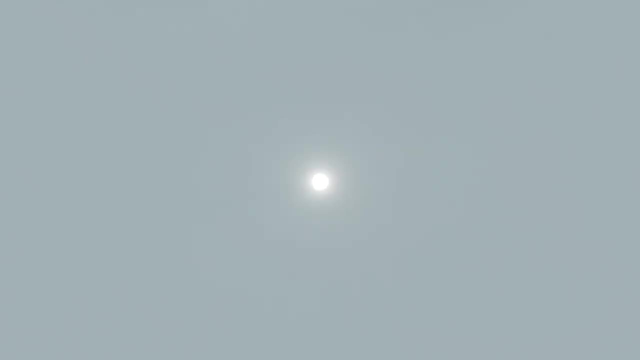 If expansion stretched out our light a thousand times over 13.7 billion years, then our solar system should have been about 75 times smaller a billion years ago. But by observing how light coming from different distances has been affected by the universe, it's. 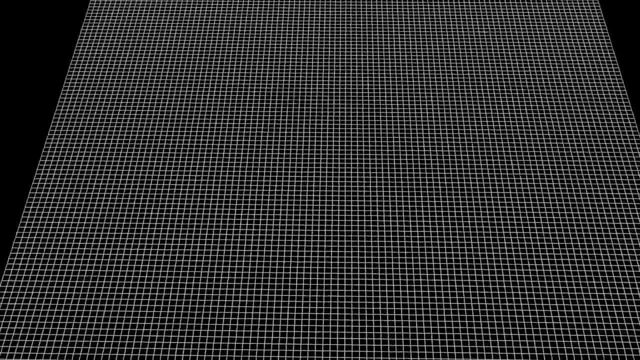 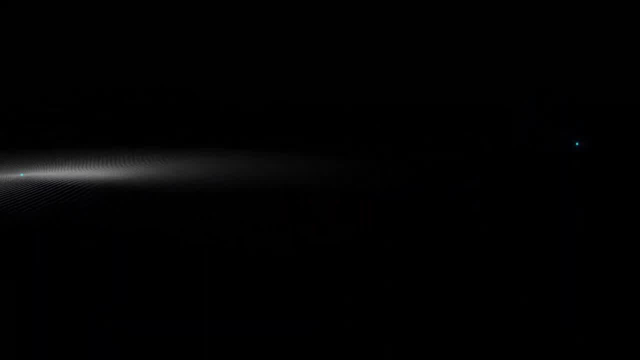 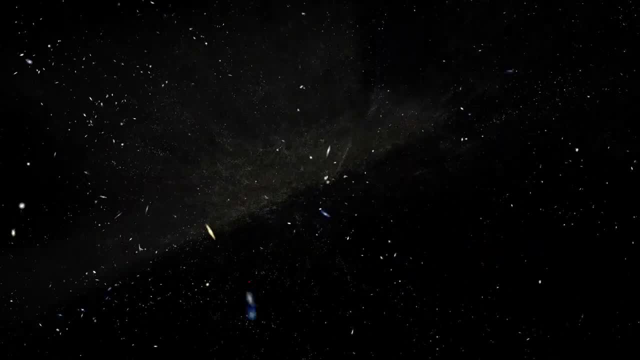 passed through on its journey. we can observe that the universe does not expand linearly. It expands faster the further two points in space get from one another. In other scales, like solar systems and galaxies, this expansion isn't really noticeable. But at immense distances, like that between far and even further galaxies, things begin. 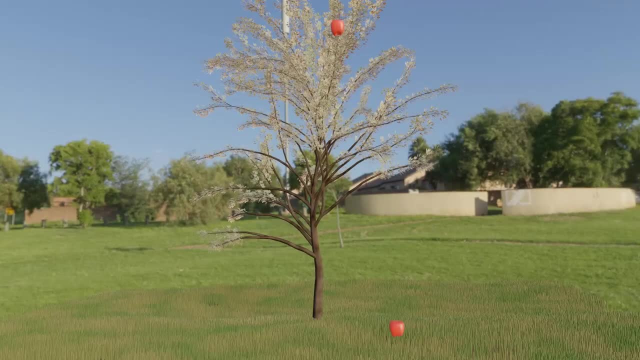 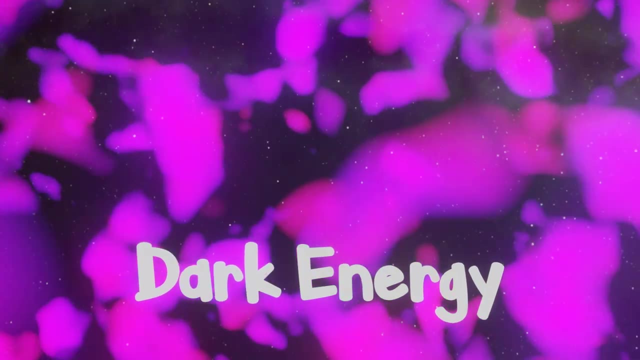 moving away from each other faster and faster, like the inverse of gravity. Now, the reasoning of this, we believe, has to do with the nature of dark energy, an unknown, relatively recent phenomenon that is not the subject of today's video. But the results. 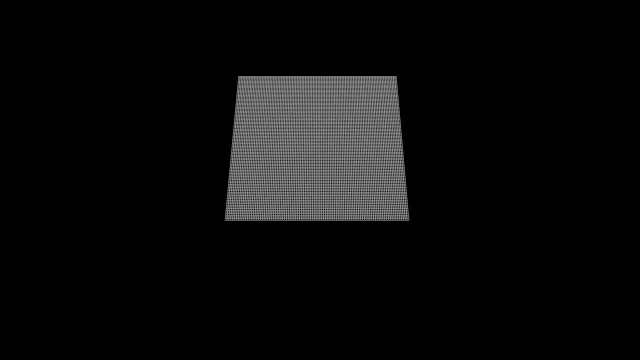 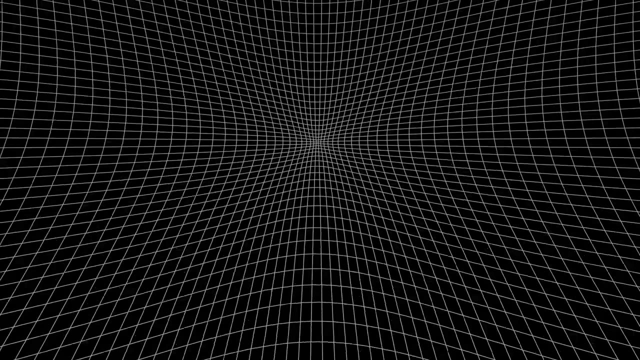 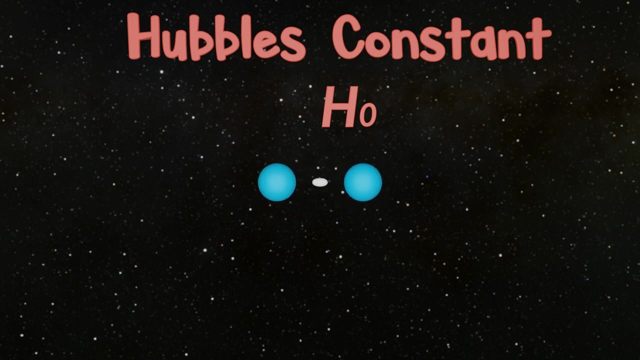 are truly strange, Since the universe is indeed expanding. the question now is: how fast and what does that look like? For this we refer to Hubble's constant. This is a factor describing the rate at which two points in space move away from each other based on their distance. It evaluates to roughly. 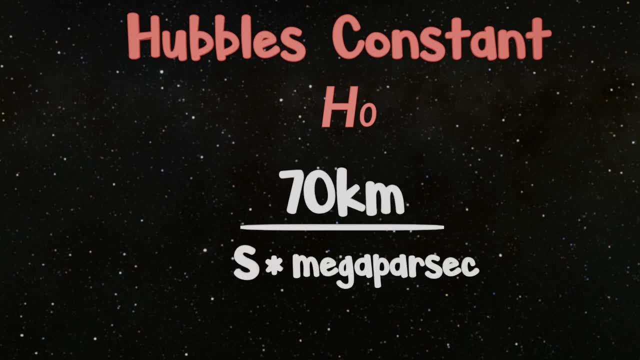 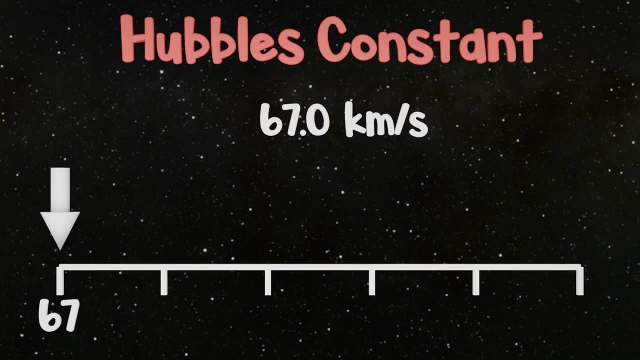 70 kilometers per second every megaparsec between the two points. This value hasn't reached consensus in the scientific community, though It wavers from roughly 67 to 72 kilometers per second. So we still have more to learn, But if it is correct, then two points, one megaparsec away, are expanding from each other. 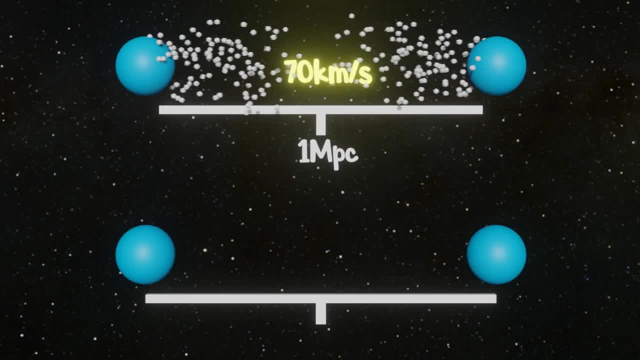 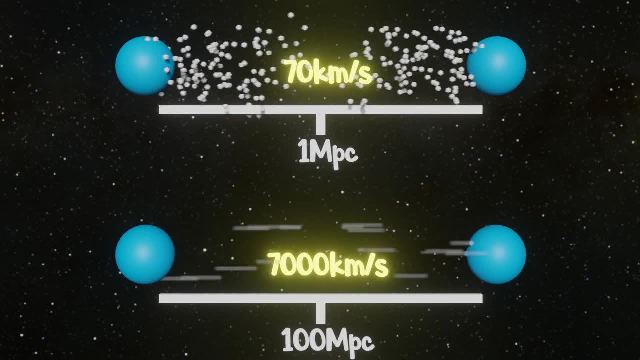 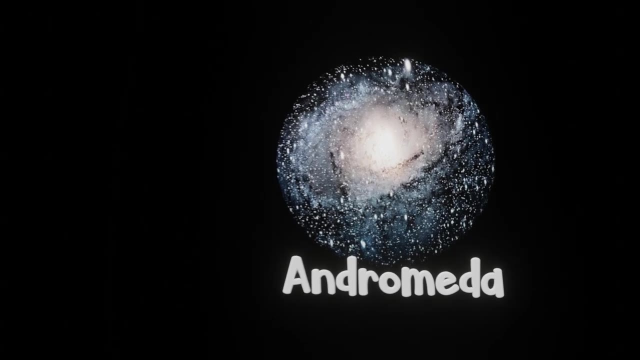 at a speed of 70 km per second, and two points, 100 megaparsecs away are expanding from each other at 7000 km per second. A megaparsec is equal to 3.26 million light years. For comparison, Andromeda, our nearest. 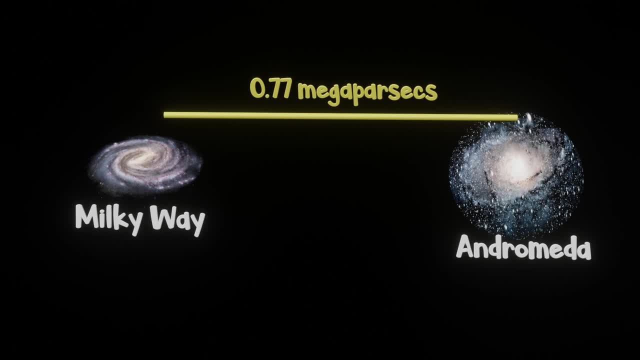 galaxy is .77.7 million light years. This gives us the next one. Our nearest galaxy, Andromeda, is .77.7 million light years. It is the nearest galaxy in the world to the 7 megaparsecs away, so there's not too much expansion happening nearby. 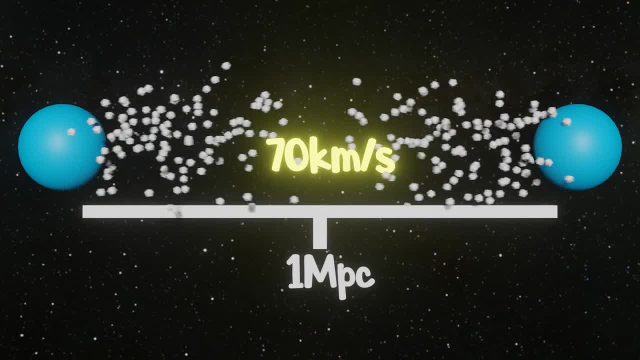 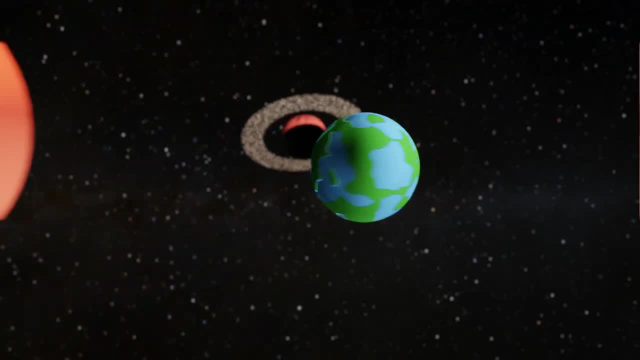 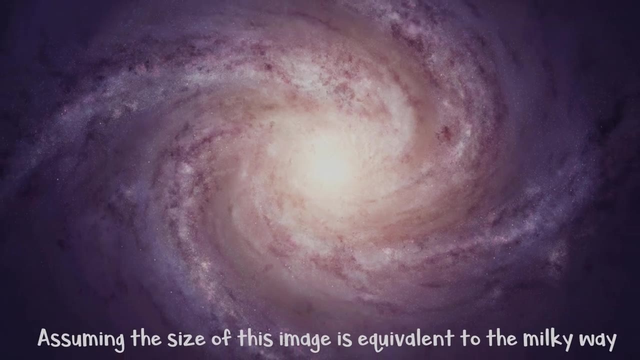 But even a megaparsec away, objects only move 70 kilometers a second. It sounds very fast, but that's only roughly two and a third times faster than the Earth's orbit around the Sun. And remember, space is very, very large. 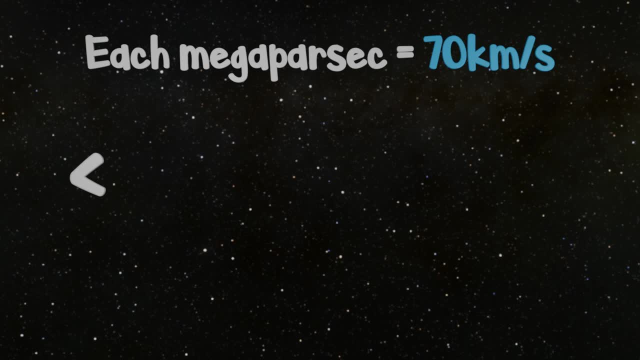 Each megaparsec of distance creates a speed of less than a quarter of a per-meal of the speed of light. An object would need to be over 4.2 billion parsecs or 13.9 billion light-years away.